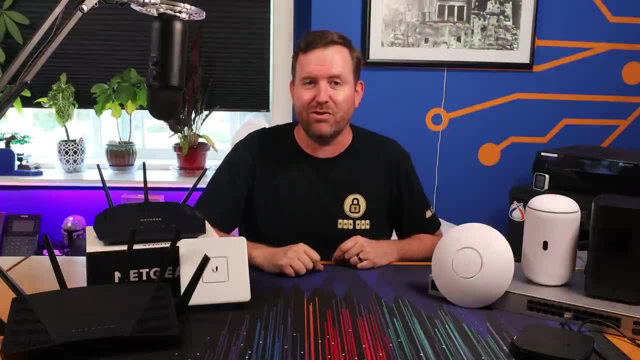 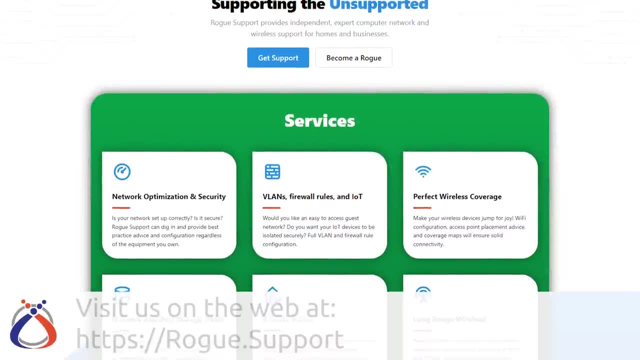 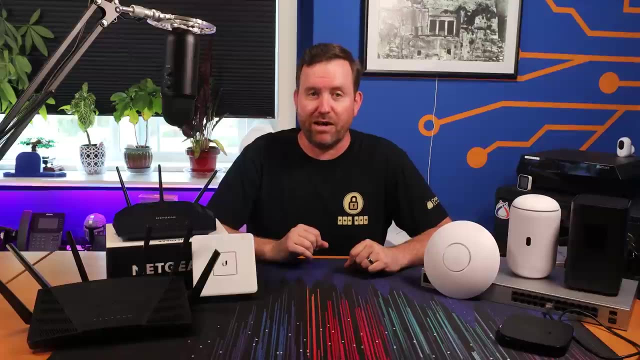 truly to provide you with the tailored assistance that you need. So, whether you're grappling with frustrating Wi-Fi signal issues, looking to set up a secure network for your guests or IoT devices, or simply seeking to optimize your network performance, Rogue Support is just a click away. 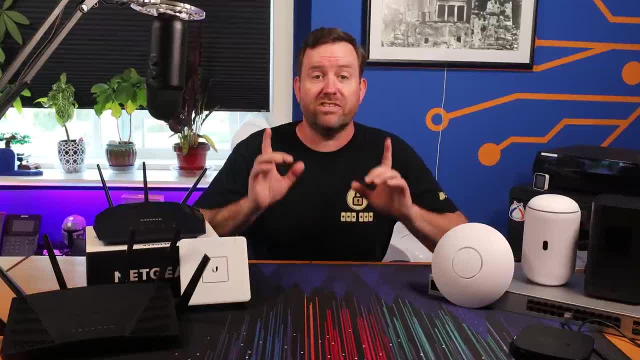 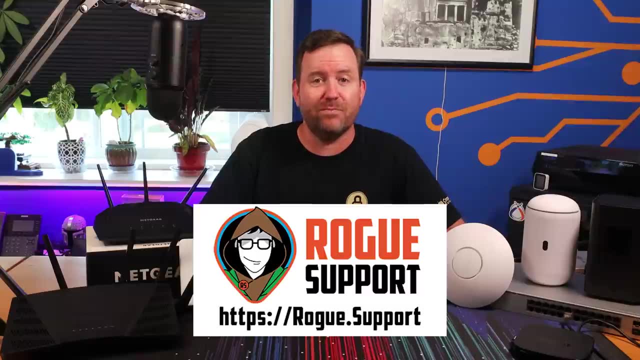 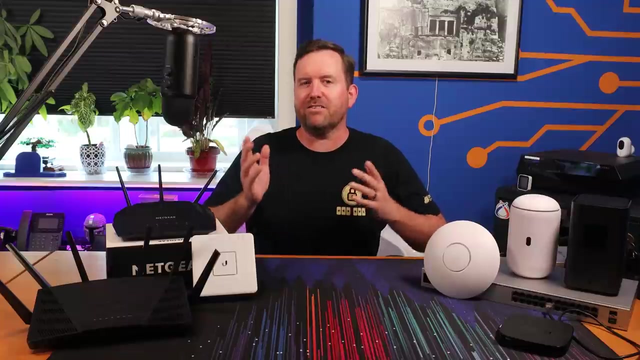 with the best of network professionals. At Rogue Support, we understand that even the best of network professionals can take on the challenges of networking. At Rogue Support, we understand that every不多 and every few people requires the resources said to fit your needs. Computer networking at its most basic is the ability for two devices to communicate with each other. If you have two, 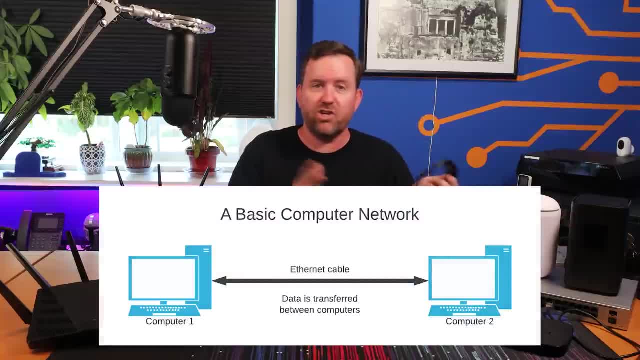 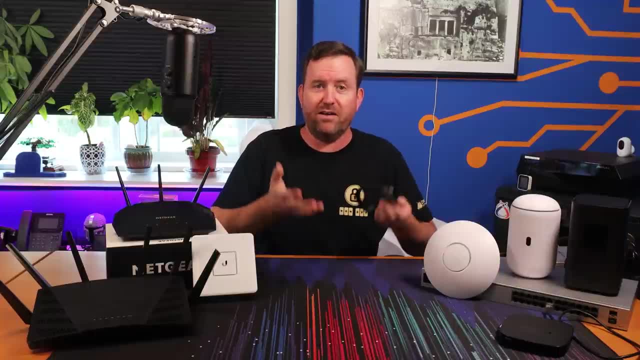 computers that are connected with an Ethernet cable and configured to share files or music or pictures of cats with each other. that's a network. Now imagine being able to share those same files, music or pictures with cats with every computer in the world. Well, now you've invented the Internet, So let's take a 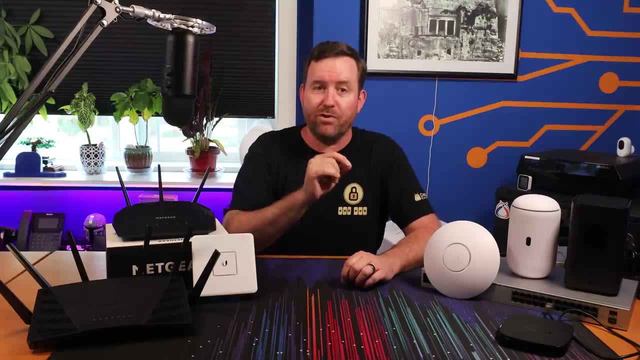 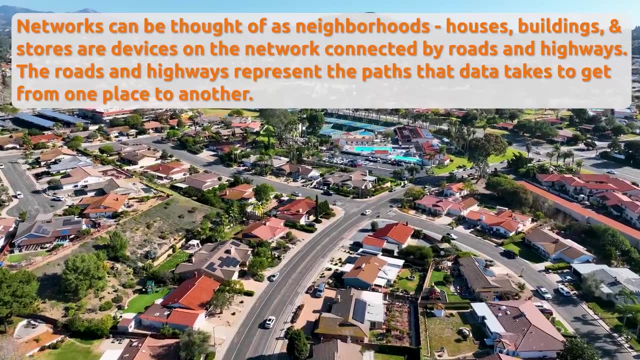 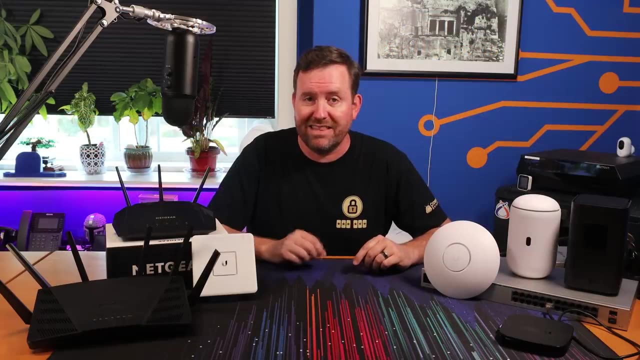 step back and think of networking in terms of your own neighborhood. In your neighborhood, you've got houses, apartments, you've got stores, a post office. Think of each of these different entities as endpoints that are all connected to each other by roads, intersections and highways. So in this 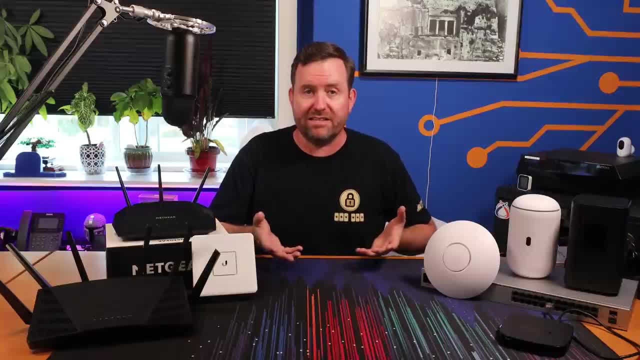 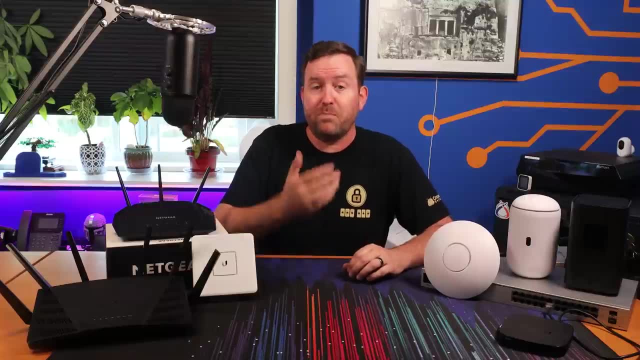 analogy, the houses and stores and buildings are all devices. Could be a computer, a laptop, your smartphone. Now, when you go visit amazoncom to do some shopping, that's basically the same thing as driving down the road to visit your local grocery store, But instead of traveling down the road in a car or 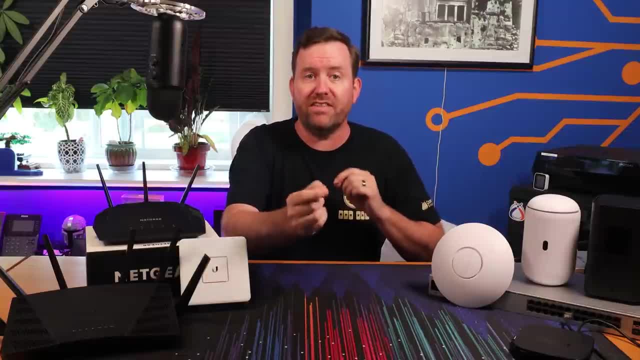 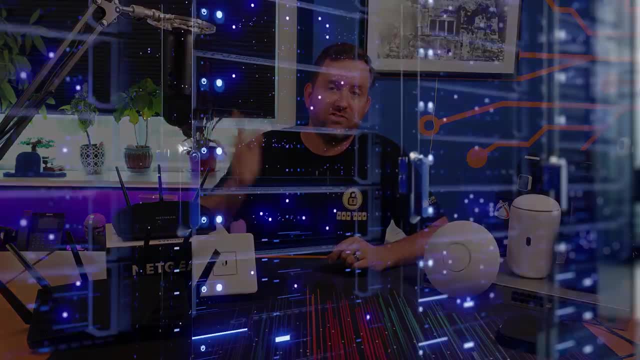 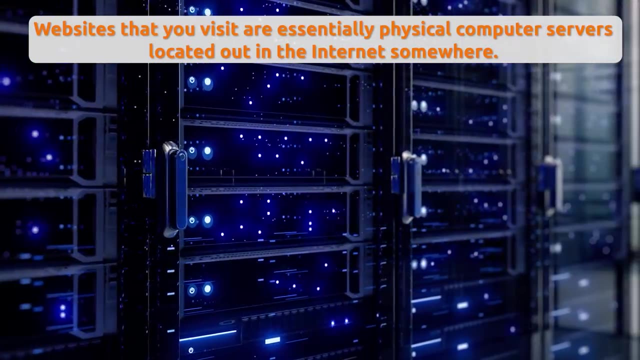 bicycle. it's your data and information traveling out to the internet and then going through many different networks between point A and point B. Websites are simply computers somewhere out in the world that are specifically designed to respond to your requests and deliver you the information that you're seeking. 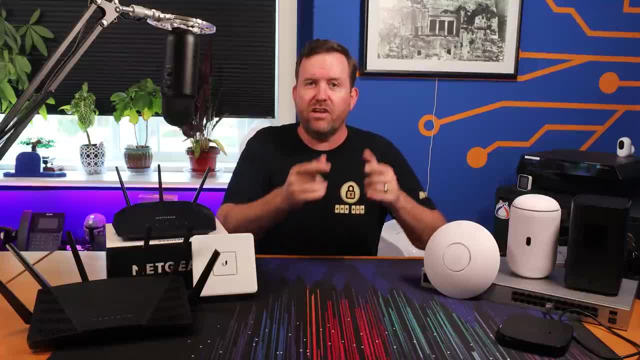 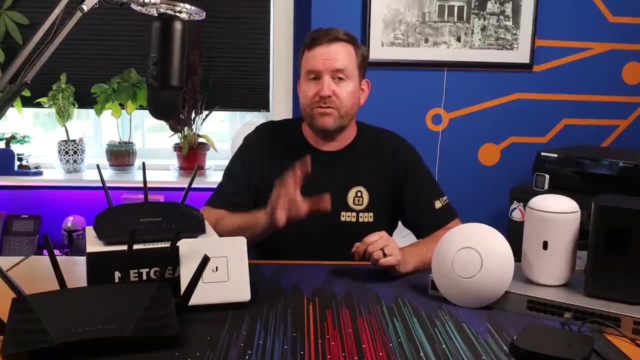 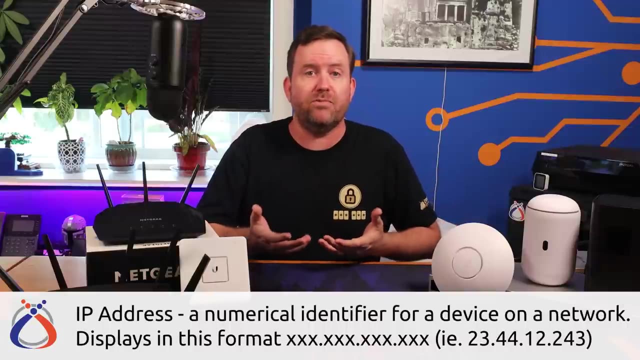 So how does your computer know to share files with another computer in your house, let alone some unknown server running a website out there on the internet? Every single device on a network has a unique identifier, which is known as an IP address. It's a very similar concept to how the post office delivers mail to your home. 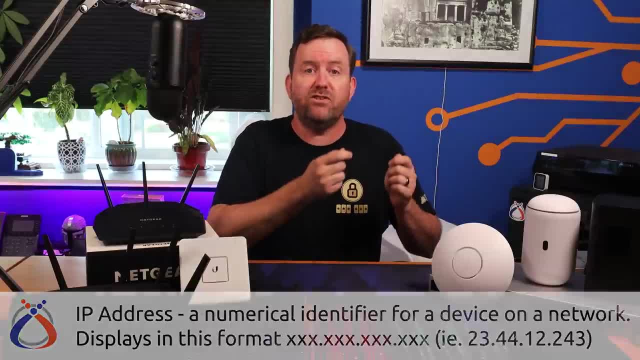 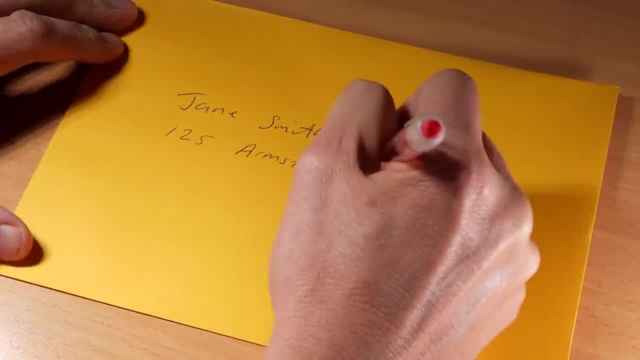 When you send a letter to someone, how does it get delivered? right, It's because you've written the destination address on that letter with a street name, number, city, state, postal code. IP addresses are like the digital equivalent of house numbers in a digital neighborhood. Using that same concept. what do you put in an envelope? You put in a letter, right, which is some data. In the real world, your letter gets delivered to the destination address, but in the digital world, your data gets delivered to the destination IP address. 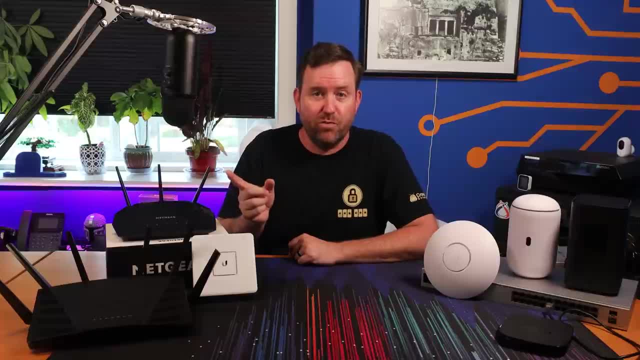 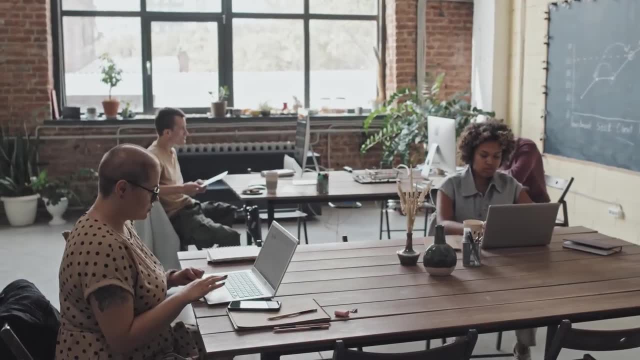 Now, whether that data needs to be delivered to a computer in the next room or to a website on the other side of the planet, the concept is the same. These digital IP addresses and highways are what allow us to send emails, stream music and movies, video chat with our grandparents, and so much more. 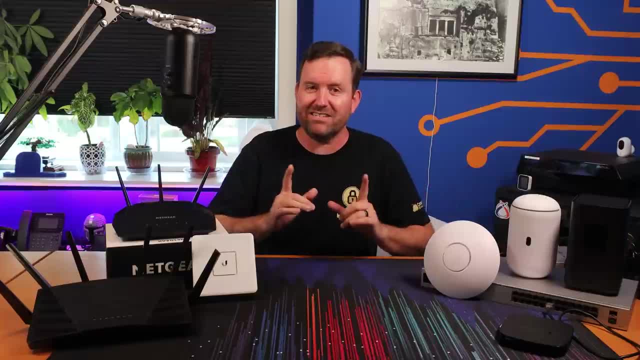 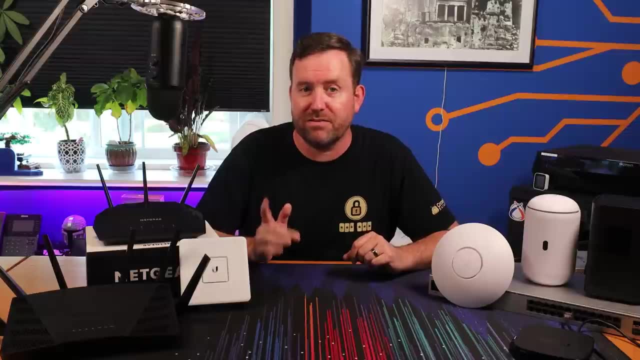 It makes this world seem a lot bigger and a lot smaller at the same time. So then, why is it important to have a well-designed home network? Well, there's gonna be many reasons for that, but to me it boils down to one simple thing. 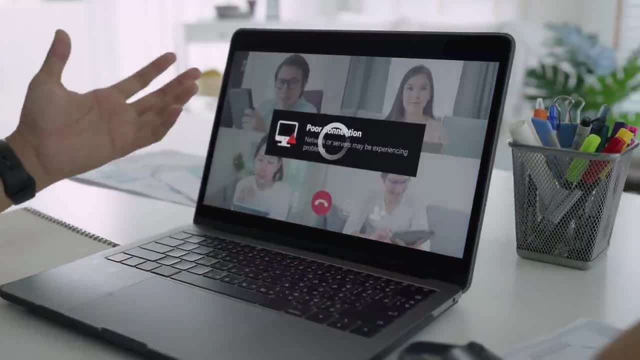 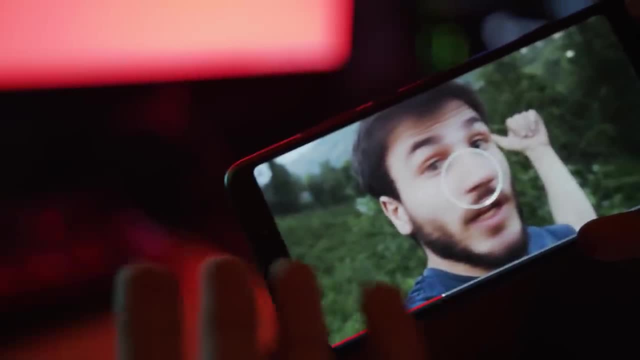 If you're having to think about your network, then it isn't working properly. What do I mean by that? Well, when you have websites loading slowly, or you can't get Wi-Fi in the upstairs bathroom, or you can't stream your favorite YouTube channel, Crosstalk Solutions, from your phone. 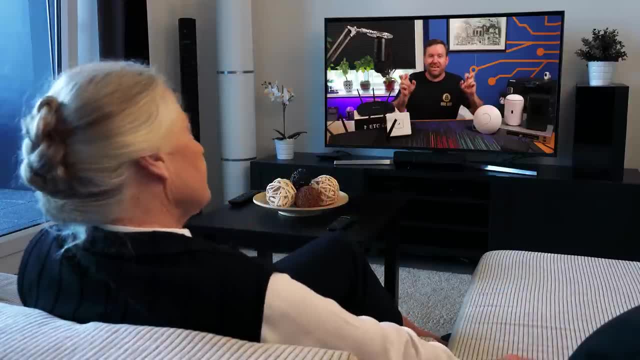 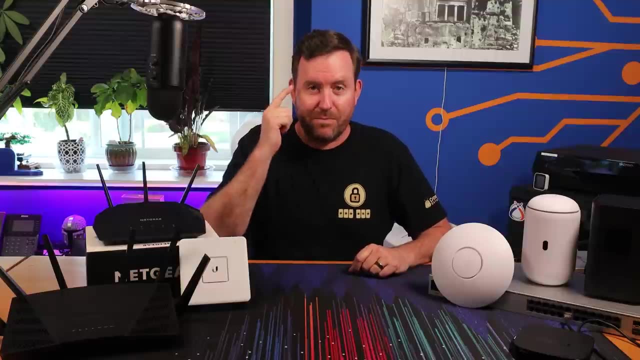 to the TV So that your significant other complains about you watching that computer guy again. Well, these are all examples of a network that isn't working reliably and you're having to think about it. right, Your network should function so seamlessly that you never have to think about it. 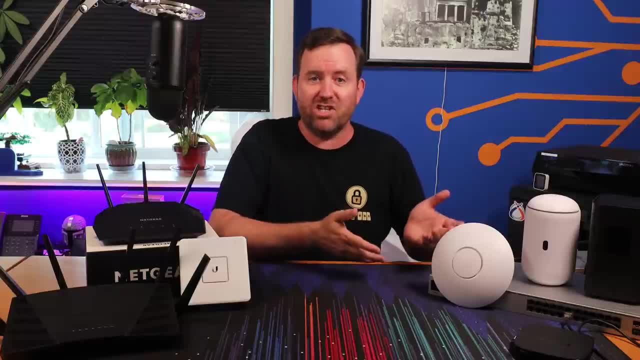 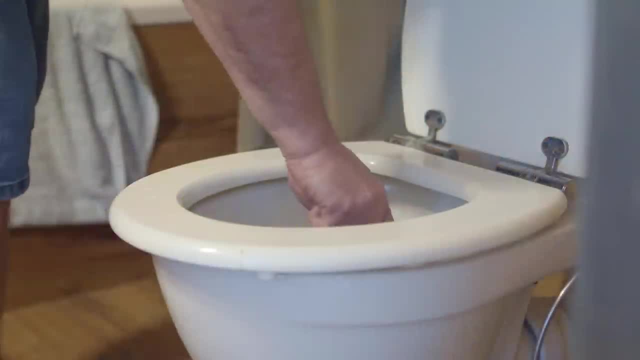 It's like the plumbing in your home: right When you use the sink or take a shower or flush the toilet and everything's working fine, you don't give it a second thought. But when the toilet backs up or the shower fills up with two inches of water, you've 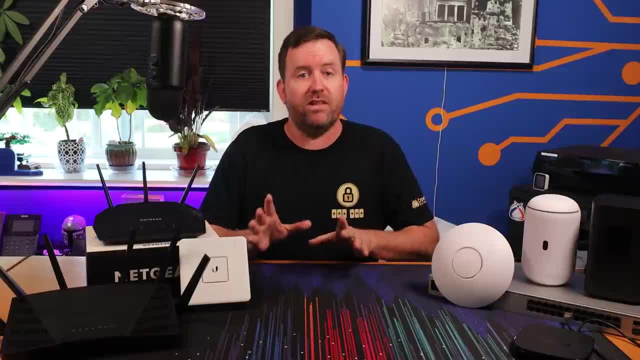 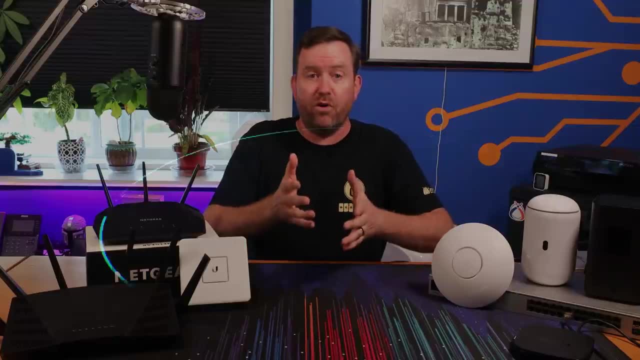 got a problem that needs to be solved. But it also goes beyond reliability right. A well-designed network means that you're going to get optimal performance out of your internet connection. I mean, after all, you're paying for a certain internet speed. 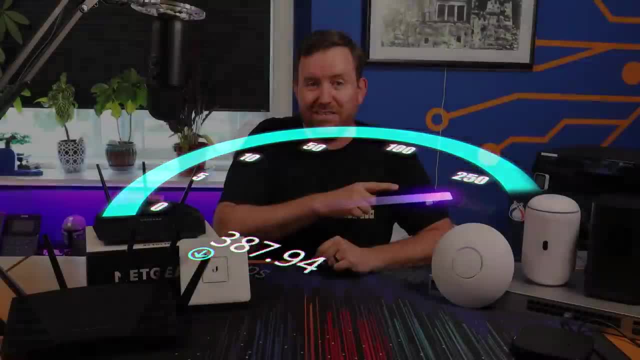 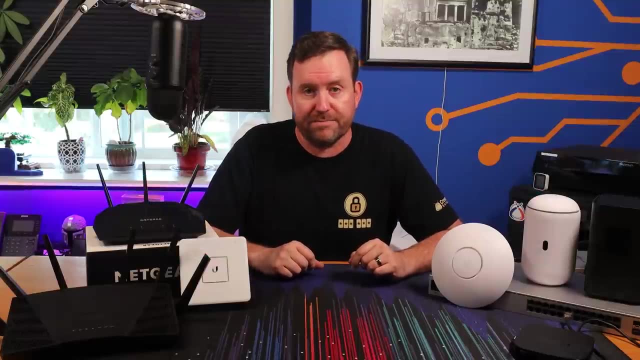 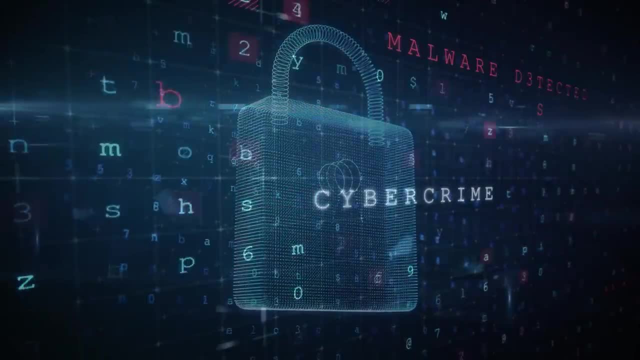 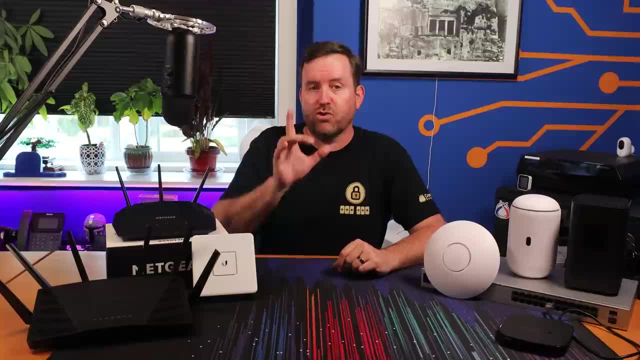 You just don't want to be exposed out to the big, bad internet, just like you wouldn't want to leave your front door unlocked at your house. Safeguarding your network and connected devices is crucial in this era, where online threats, identity theft, malware- these are all serious issues. 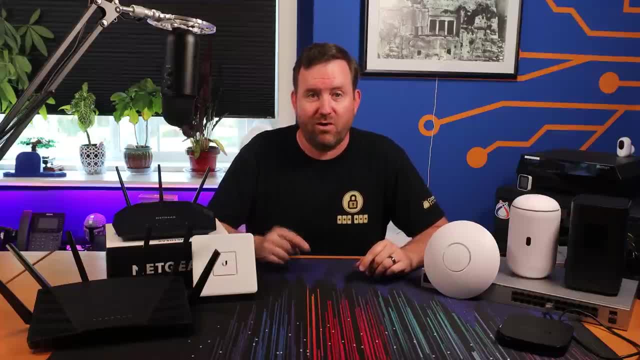 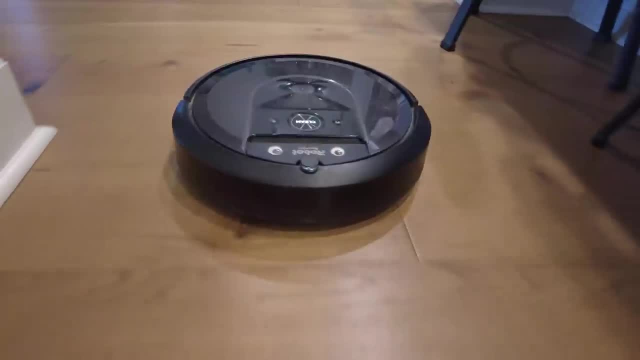 We're definitely going to spend a lot of time talking about securities and firewalls in this series. Finally, a well-designed network is future proof. Now, 10 years ago, I never thought that I'd be controlling my robot vacuum with my smartphone. 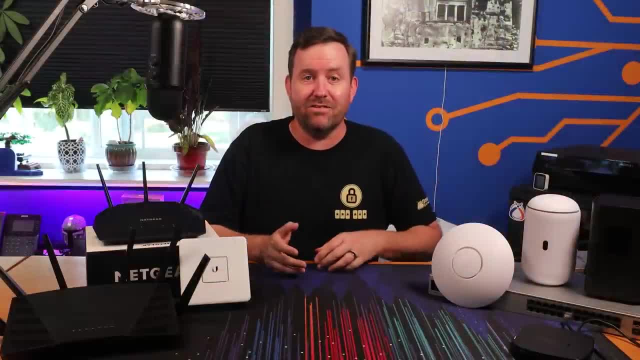 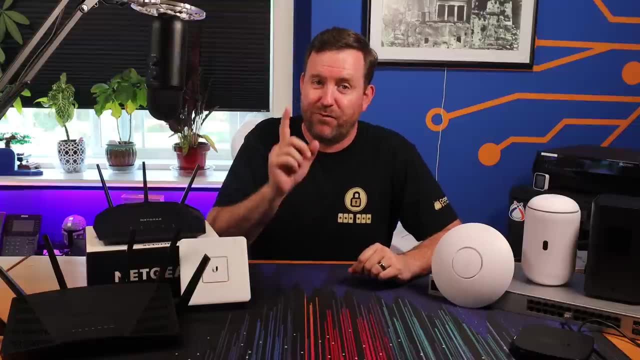 right. But here we are. we're going to be in the next 10 years. By investing some time and effort into your home network, you're going to pave the way for a reliable, high-performing, secure and future-proof digital environment. Now let's dig into the basic components of a computer network that you're 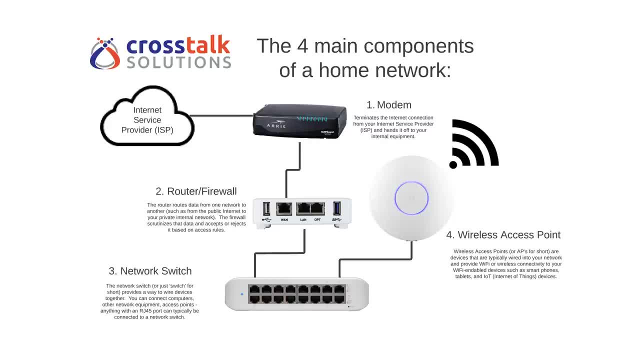 likely to run into as you design your own system. There are four main components to any home network: the modem, the router, firewall, network switches and wireless access points. Now we're going to dig deeper into each one of these components individually later on in the tutorial series. 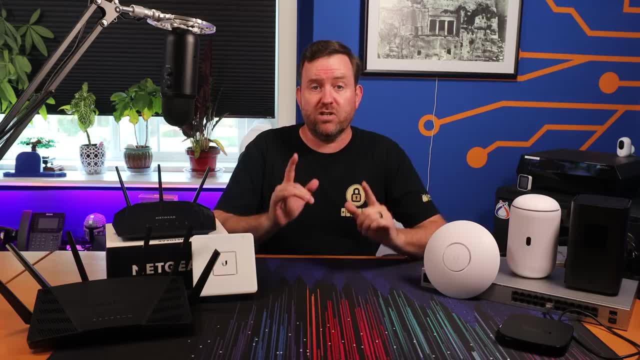 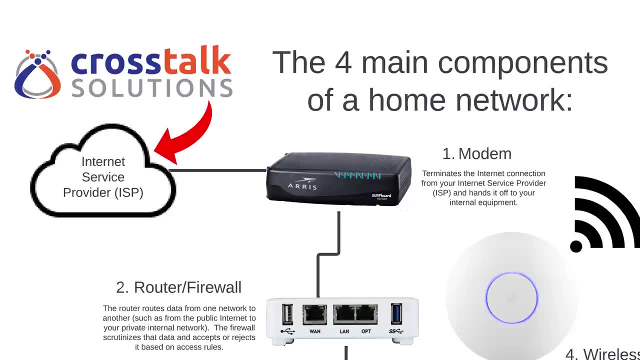 but let's do a brief overview, just to get started. The first device you should be aware of is the modem. When you sign up for internet service from an ISP or internet service provider, whether that connection is fiber internet, cable, DSL or even satellite internet such as Starlink, the ISP has 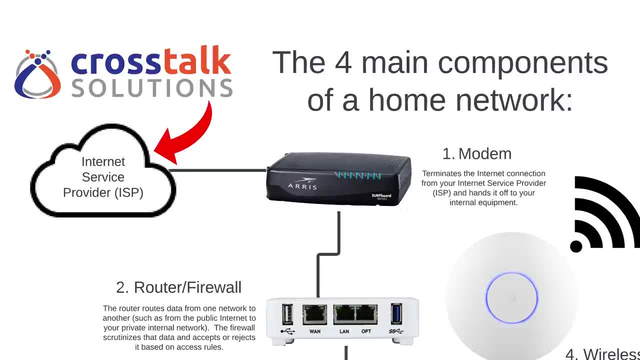 to give you that connection so that you can use it somehow right. And typically the piece of equipment that they give you to handle that connection is the modem. So if you're using an ISP or internet service provider, the modem is the bridge between your home network and the 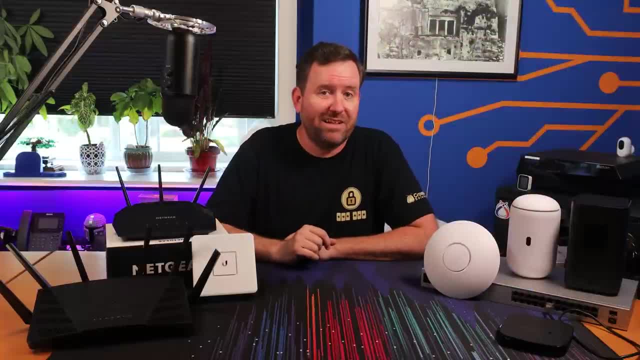 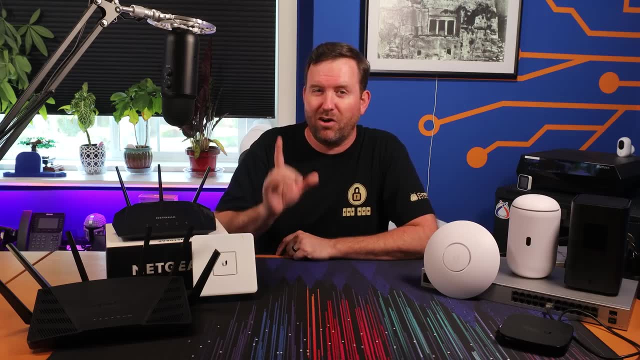 internet service provider. The next piece of equipment you'll typically see is a router or firewall. Now, technically speaking, a router and firewall are actually two different things, but they can also be used pretty interchangeably. A router is simply a device that routes traffic from. 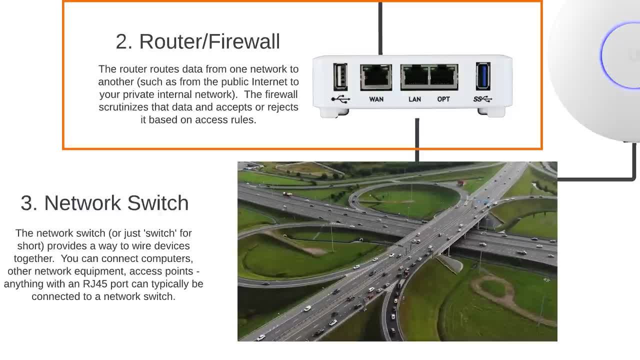 one network to another, just like driving through an interchange that takes you from one highway to another. The router is the bridge between your home network and the internet service provider. So if you were to drive through a home network, the router is actually the bridge between your home. 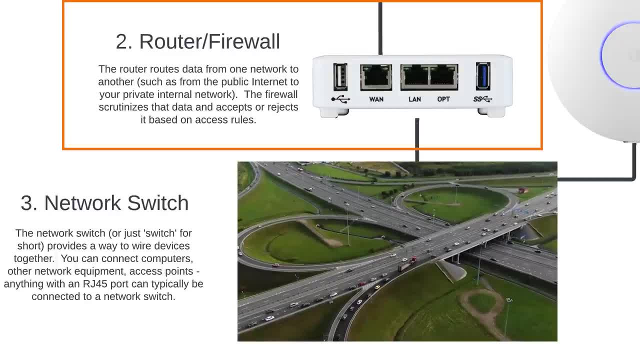 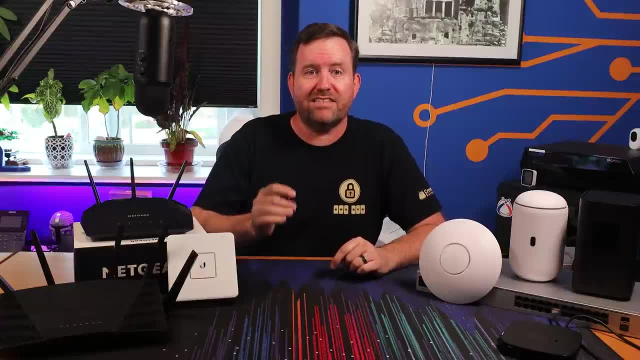 network and the internet service provider. And this is what it does. It can connect your network and it can send your data from one network to another, depending on the destination. Most often, with home networks, the router is the device that routes private traffic in your home network also. 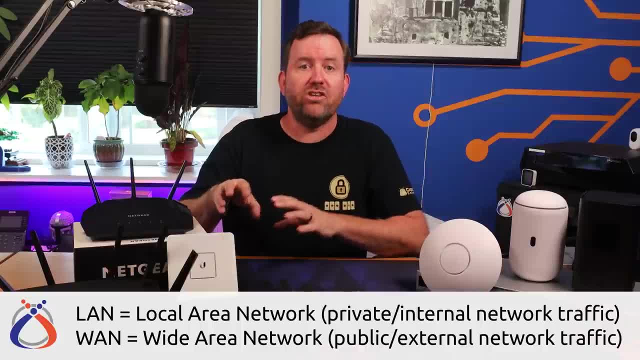 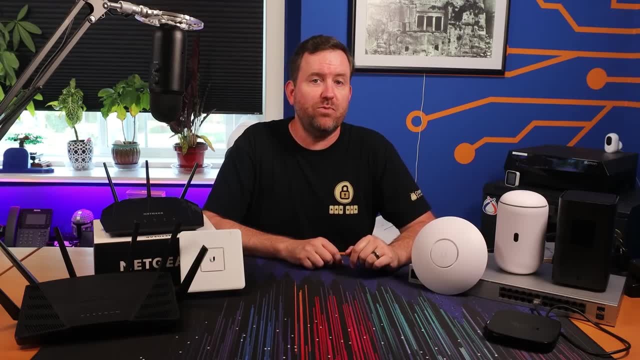 known as a LAN or local area network, into the internet or public network, which is also known as the WAN or wide area network. Lots of times, when you buy a router, it will have ports on the back labeled WAN and LAN- That's what these are called, And you can send your data from your home. 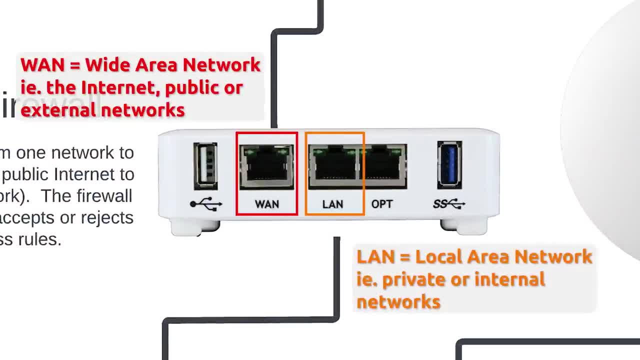 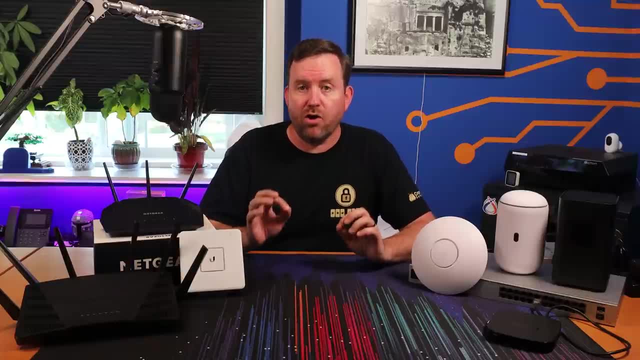 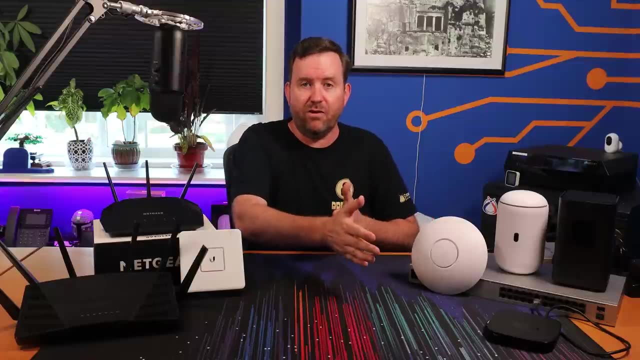 mean LAN is your private internal network and WAN is the internet connection or public network. As I said earlier, a router and a firewall are two separate things, but they can be used fairly interchangeably If a router is like the interchange between two different highways. 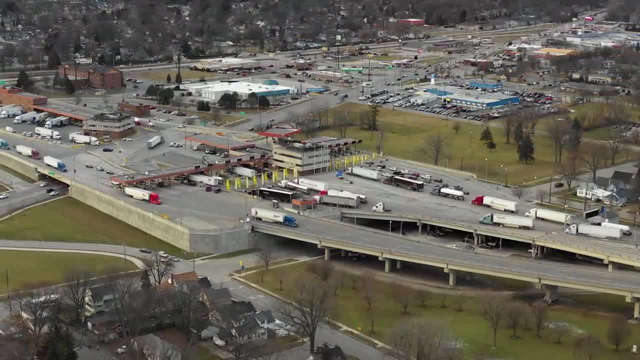 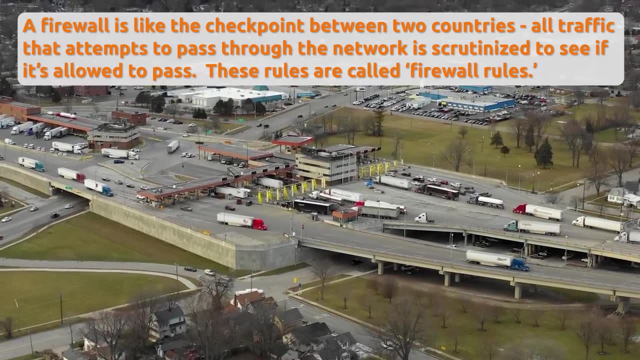 you can think of the firewall as a checkpoint on a highway between two different countries, right? So here in the US, if I want to drive up to Canada, I can't just drive through without stopping. There's a checkpoint that I have to pass through. At that checkpoint they're going to see if I'm allowed to. 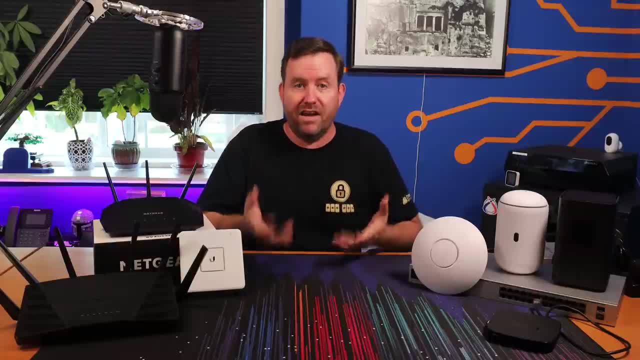 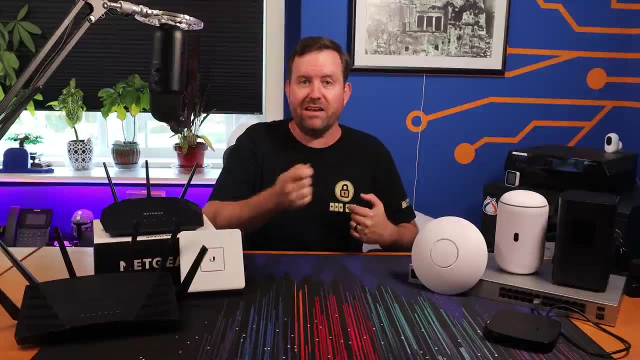 enter Canada. right, If all my paperwork's good and I've got an up-to-date passport, then I am allowed through. But if I fail these requirements, I am turned away and not allowed to enter the country. That's what a firewall is right. It's a device that has a set of rules. 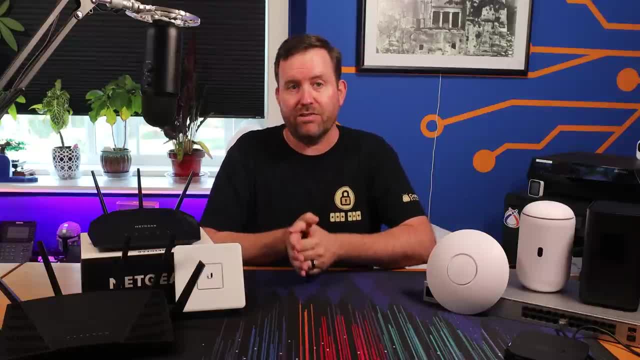 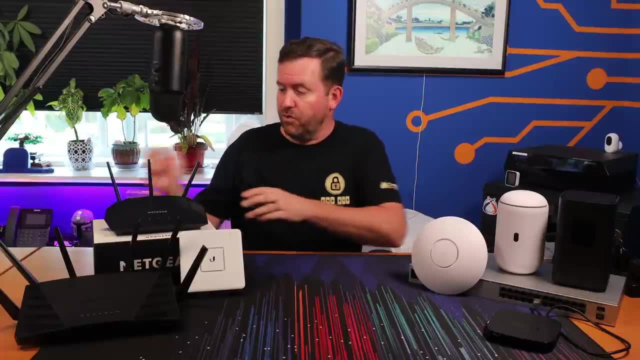 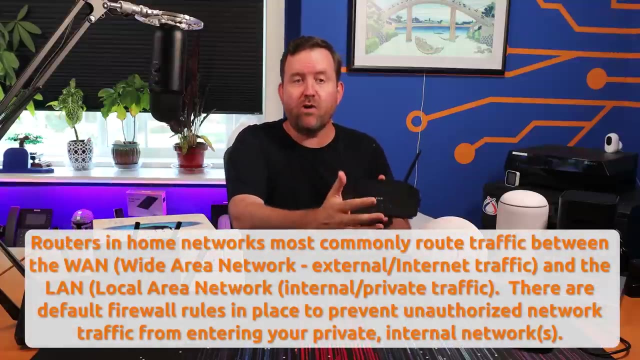 for which traffic can and can't enter a particular network. When I say that a router and firewall can be used interchangeably, this is because quite often in home networking, the router is managing the connection between your internal private networks and the internet, And that router has firewall rules in place by default that are designed to 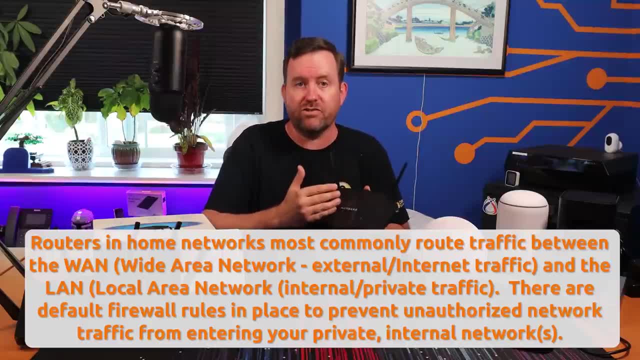 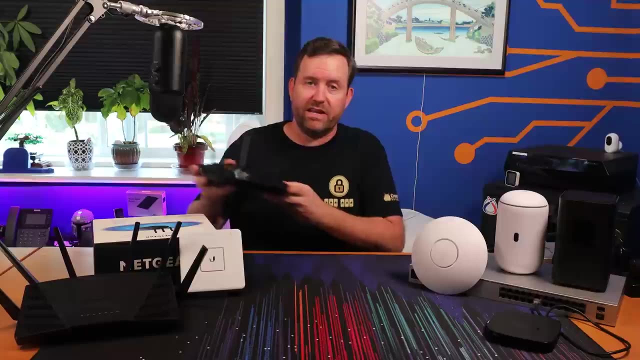 prevent unauthorized traffic from getting into your private network. So while a router can technically only be used to pass network traffic between networks without actually scrutinizing anything, a firewall is a router that has at least some basic rules set up for which traffic can pass through. So the first piece of equipment that you are likely to encounter is a network switch. 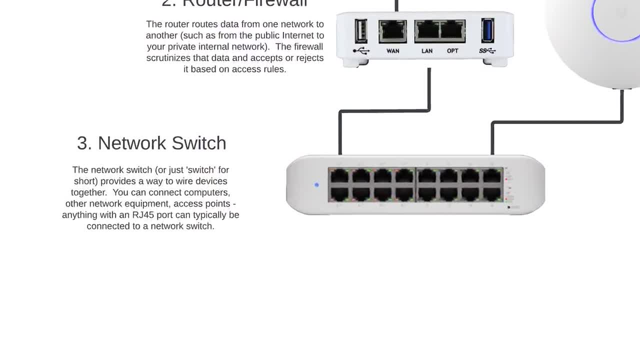 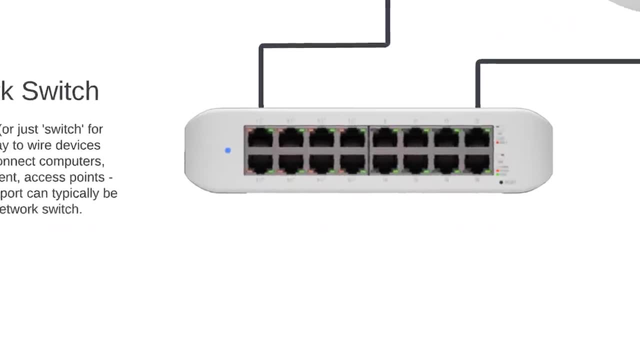 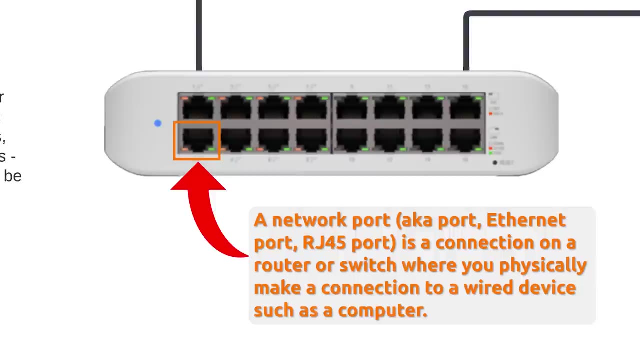 or just switch for short. So a switch at its most basic is a device that expands the number of ports available to plug wired devices into. A port is the connection on a network switch where you plug in an ethernet cable. So any device that has an ethernet connection, such as your computer. 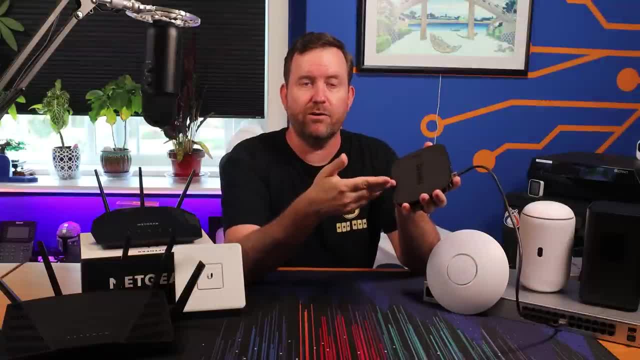 your smart television, your Xbox, PlayStation or, like this, Roku right here, can be connected to a network switch. So a network switch is a device that's connected to a network switch. connected to the switch with an ethernet cable. You plug one end of the cable into your device. 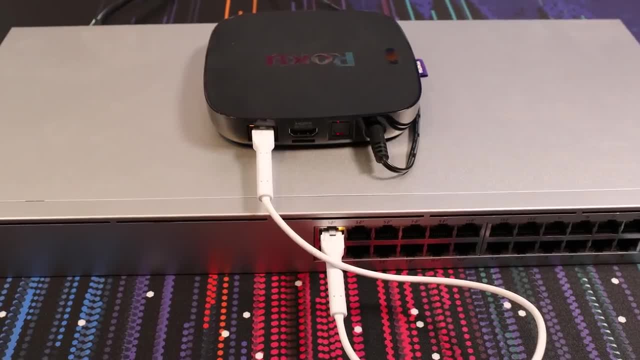 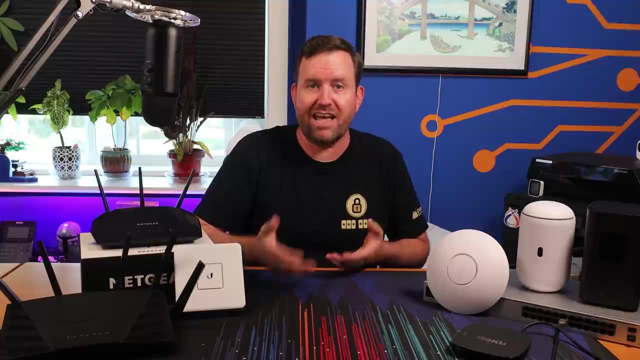 and you plug the other end of the cable into the network switch. When you run out of switch ports, you can simply add another network switch to the network, or you can buy a new network switch that has more ports available. Network switches can be very simple devices, but they 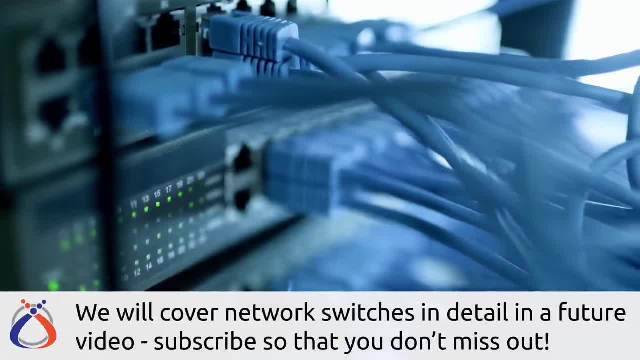 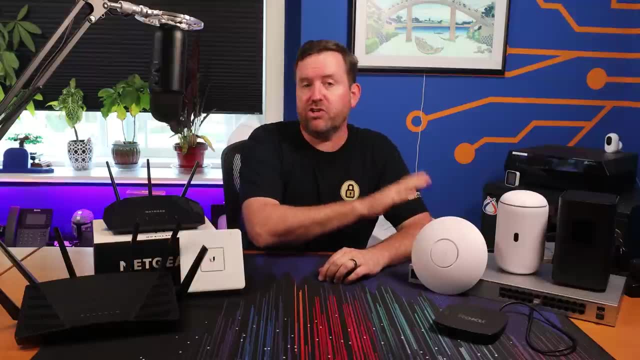 can also be pretty smart, And we're going to be discussing network switches and what they can do a lot over the course of this tutorial series, But for now, just understand that switches are mainly used to connect wired devices so that they can share data with each. 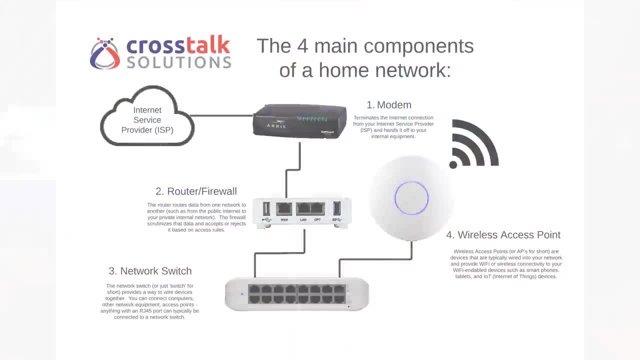 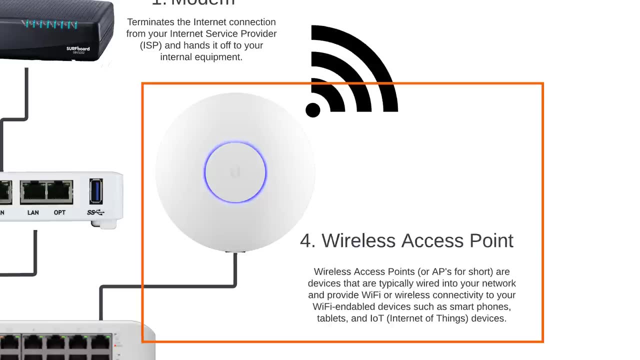 other. Let's now talk about wireless access points, or APs for short. So APs are devices that are designed to connect wireless devices to your network. They're kind of like network switches, but rather than using an ethernet cable to connect a computer to the network. 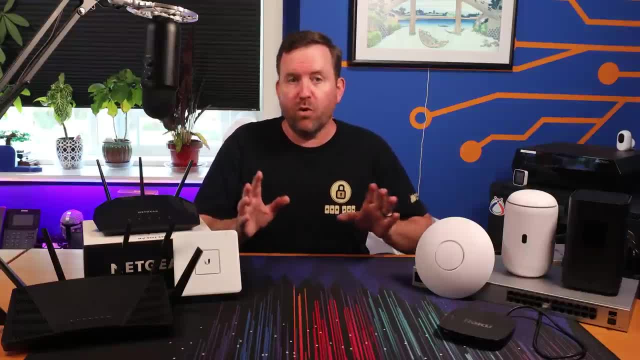 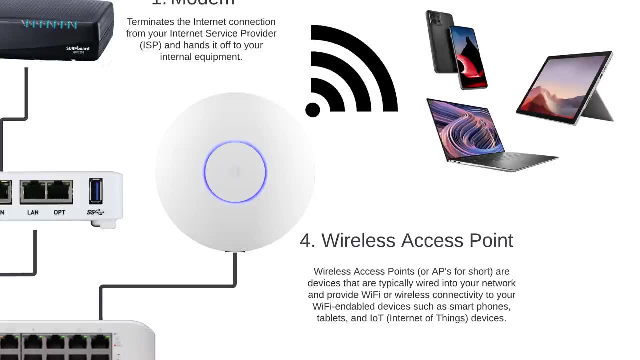 you're connecting that computer wirelessly. More and more devices these days use wireless, which is also called Wi-Fi, to connect to your network. Your smartphone, tablets, laptops and many different smart devices, like your robot, vacuum, smart switches and smart light bulbs, communicate wirelessly with an access point. 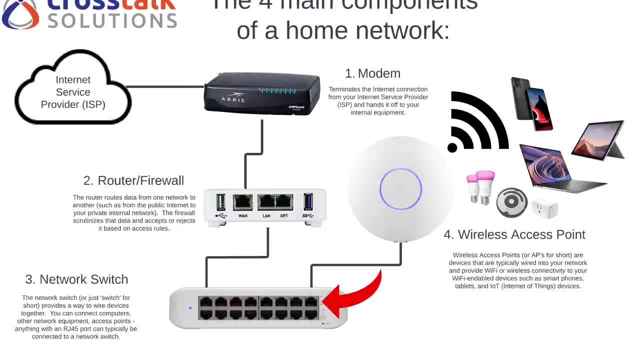 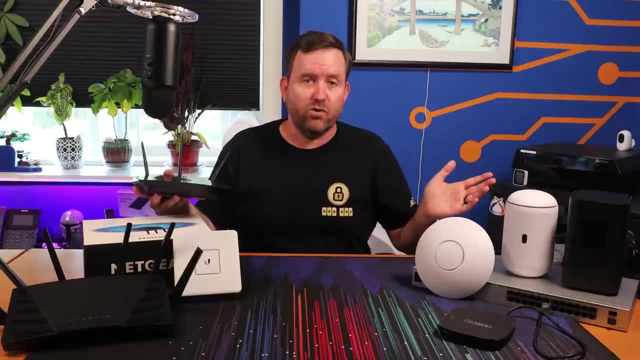 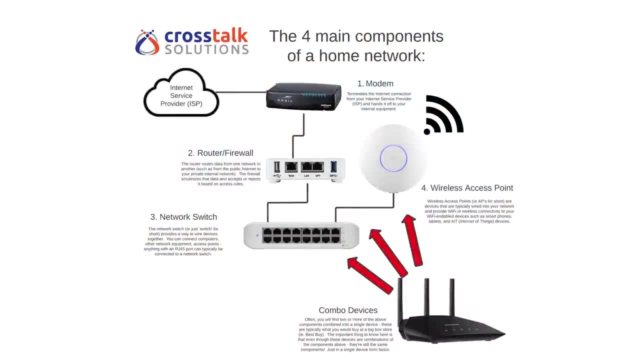 which is then connected to the network itself, usually with an ethernet cable or integrated into a combination device. Now in this series, we're going to dedicate a full video to wireless technology and how to optimize the Wi-Fi in your home for the best performance. Speaking of combo devices, here's one of the 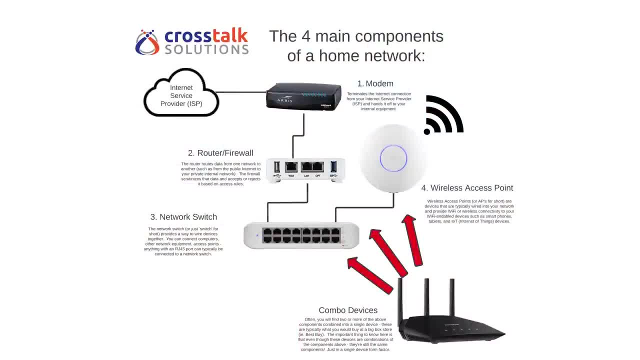 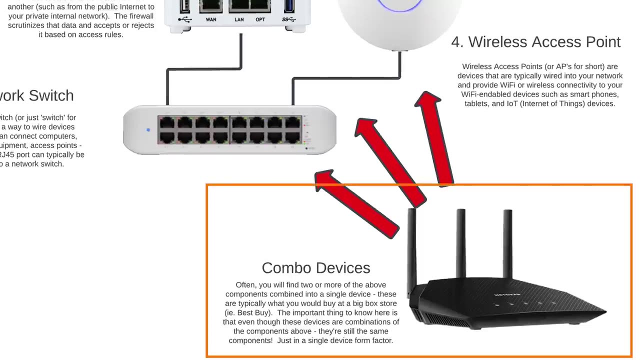 key takeaways for this first intro to home networking. In this video I'm discussing each of the core components of a home network individually, but quite often you will have two or more of these core components combined into a single device, But understanding them individually. 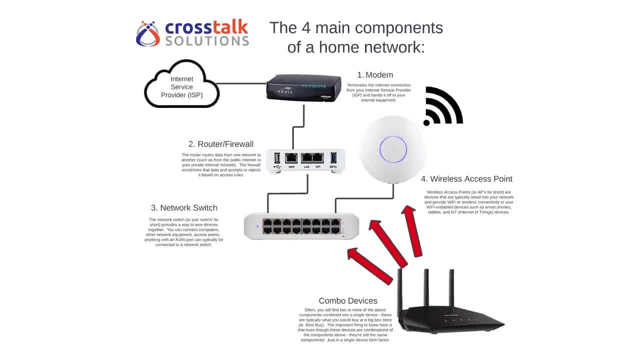 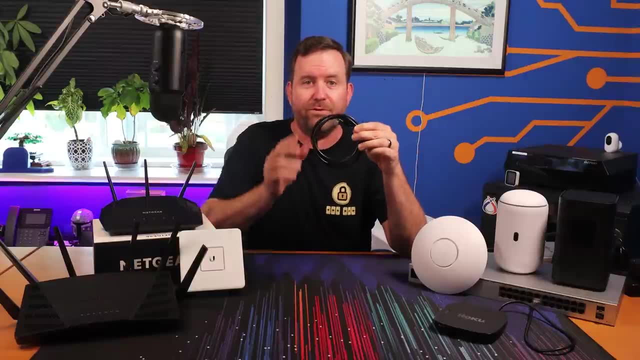 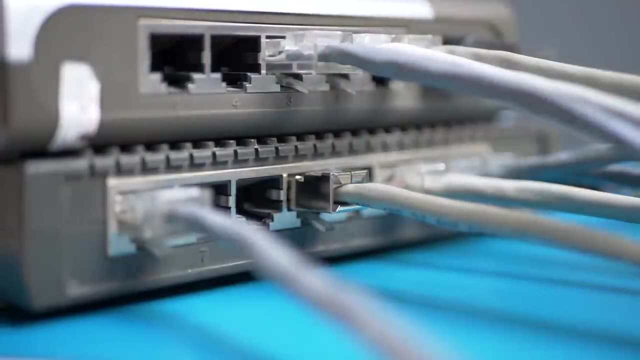 is paramount to understanding the role that any device is playing in your home network. One more thing that I should mention, that you're definitely going to run into, is ethernet cables. Ethernet cables are used to connect network devices together, such as connecting your router to the wireless access point or your computer to a switch. Ethernet cables have what's known.